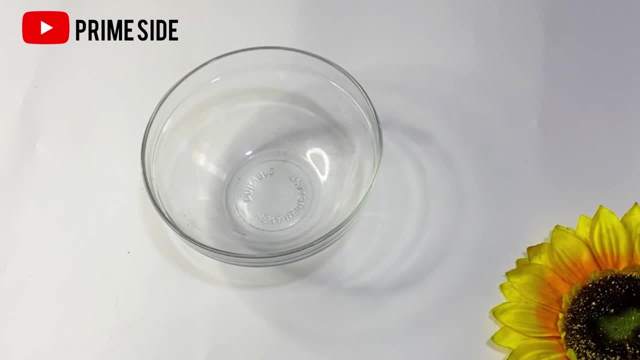 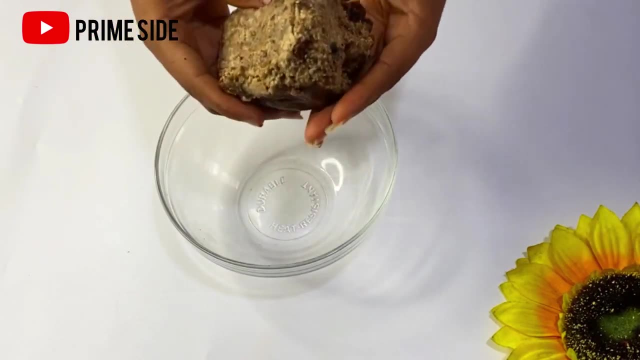 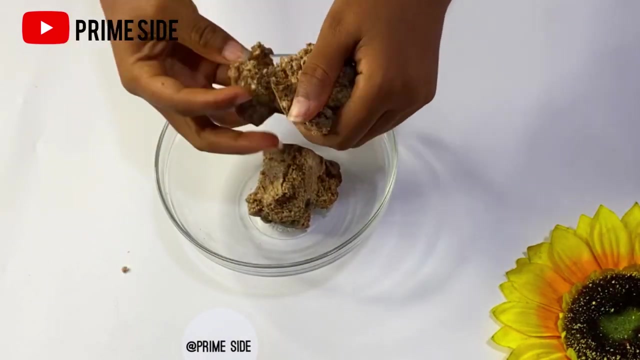 although some people call it the Nigerian soap, but, however, we usually call it the Ghana black soup as the base. This Ghana black soap is filled with so many nutrients and minerals, natural vitamins, that is suitable for the skin and suits all kind of skin. We'll be using just 100 grams. 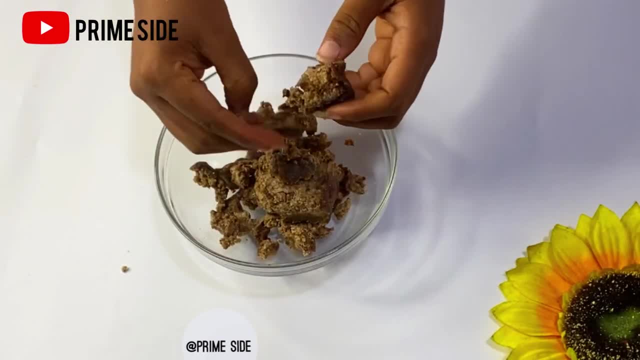 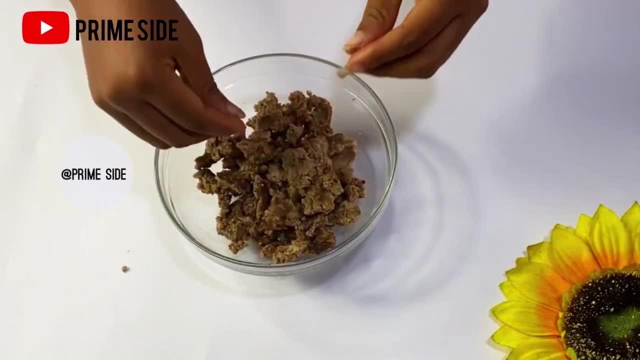 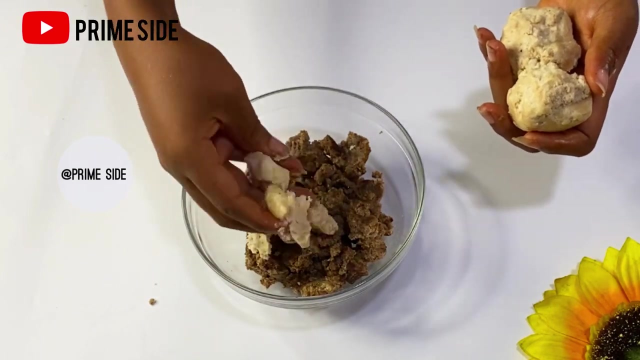 of this soap base here. Many people even use this soap alone, so mixing it with other ingredients will only help to boost this effect. and perhaps for a precise use, I'll also be using three ball soaps for my tea. I'll be using three white ball soaps, or white Ghana soaps, as you may call it. 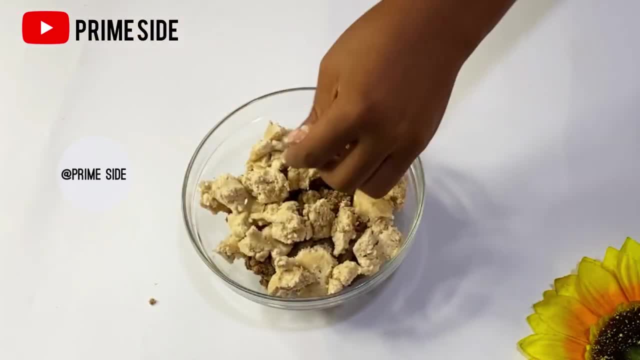 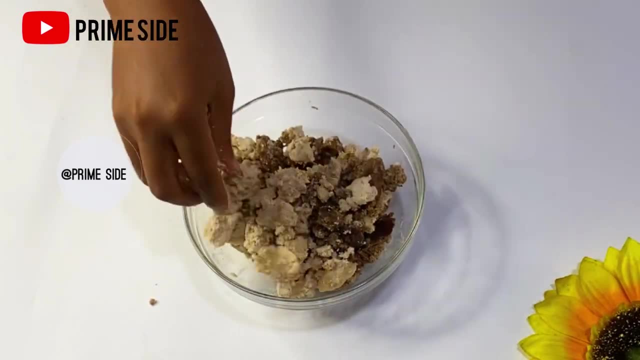 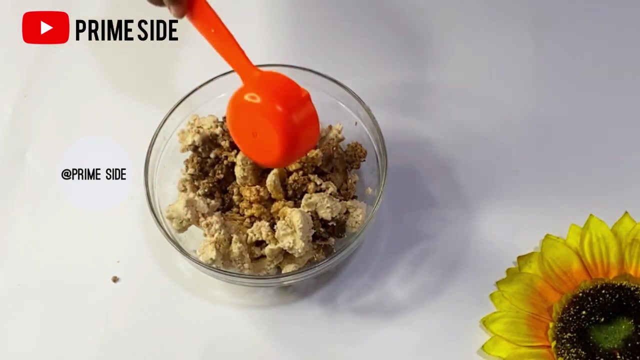 These soaps are also rich in nutrients and minerals, and they also help our soaps to lather very, very well. Into these soaps I'll be adding my Habal soap, which I also call Omiyaru. This soap contains so many nutrients and it is gotten from the residue of making the normal black soap. I'll also be going. 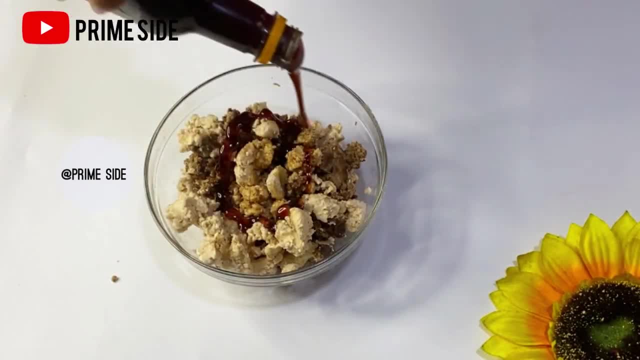 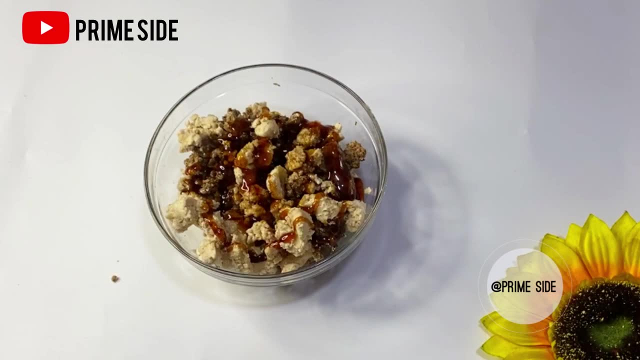 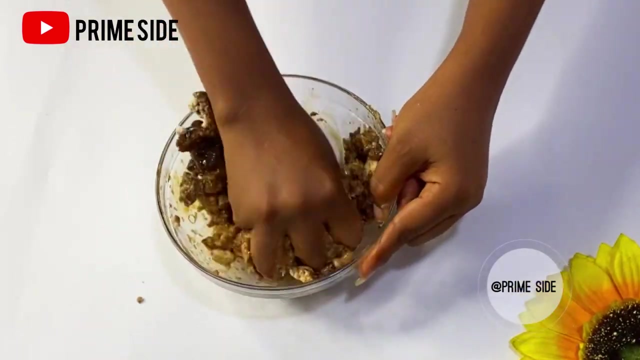 with a little bit of my natural honey. these children, they need this honey in their soup also. i'm going to be massaging with my hand. note that i didn't use a mortar and pistol for this, because it's actually a small quantity and i can actually get it mashed with my hands now also. 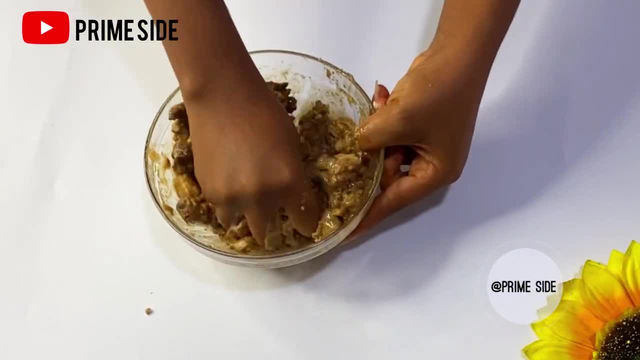 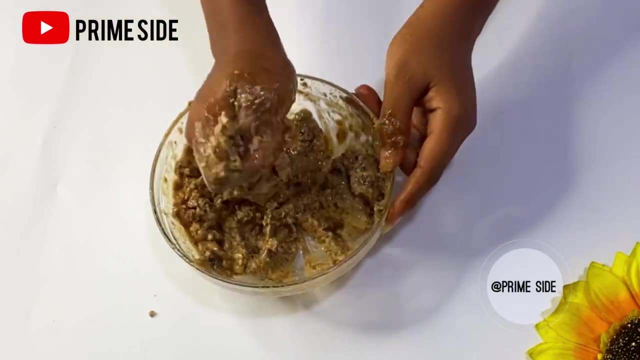 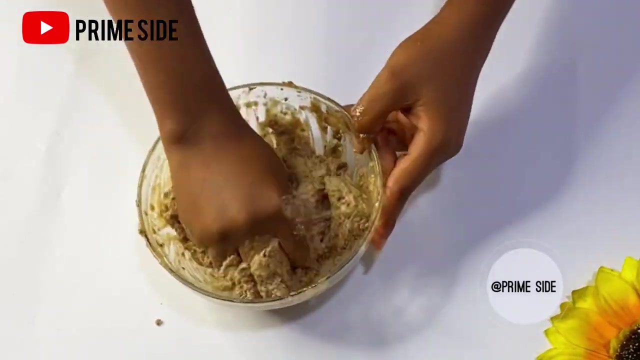 note that children do not need too much ingredients in their black soup because they are not fighting anything like acne or pimples or whatsoever, so what they are only looking for in your skin is how to make their skin soft and smooth and radiant as well, and those who want to have a top-up glow. 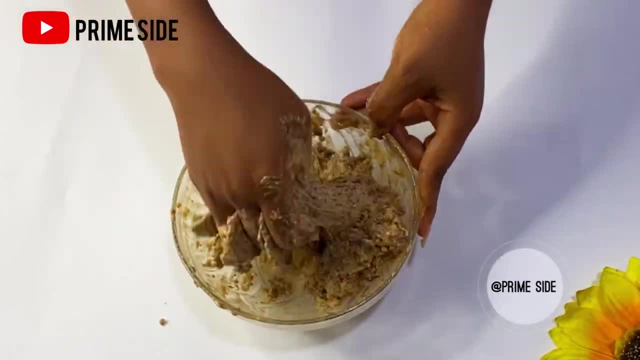 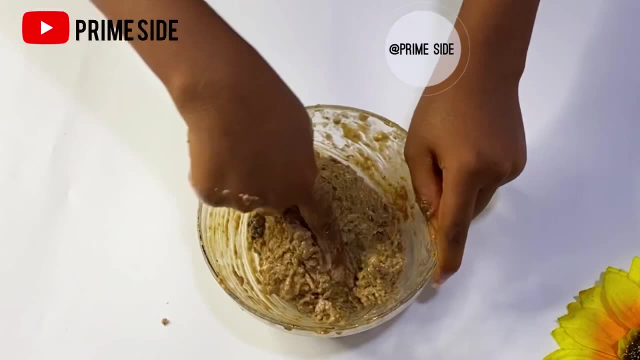 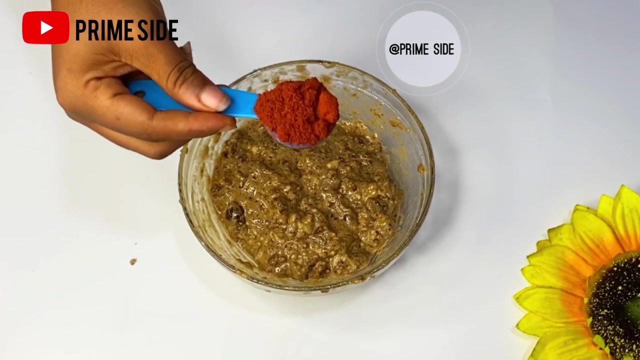 you can also use this recipe, but adding chemicals to tone the skin for this recipe is a no-no. so after mashing to this point, i'm going to be adding my powders, a very few powders that will just be suitable for your skin. the first here is the calm wood powder. i'm adding just a tablespoon. 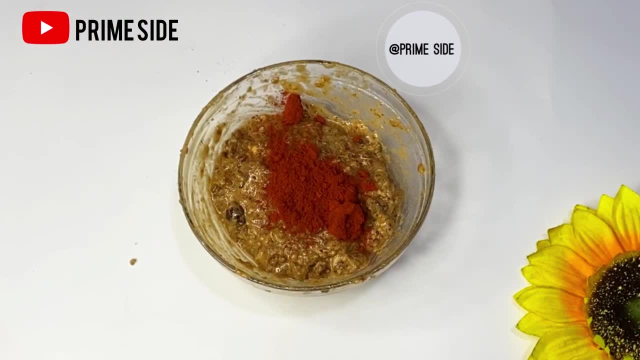 of calm wood powder. calm wood helps to brighten the skin and will also help to fight rashes on the skin. it will help to get rid of wrinkles, thereby making the skin smooth and making the child look more younger, radiant and looking more beautiful. it will fasten the soup to make. 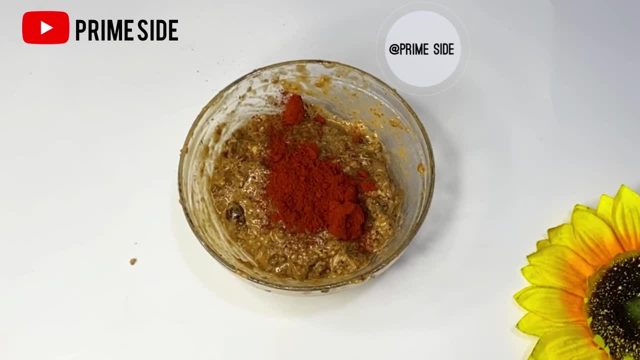 the child's skin glow and looking more radiant. the next powder we'll be adding here is our neem powder. neem powder is packed with a lot of antibacterial and antifungal properties that will help to fight this kind of conditions in this children's skin, like ringworms, rashes, rough skin, dull skin and a whole lot more. 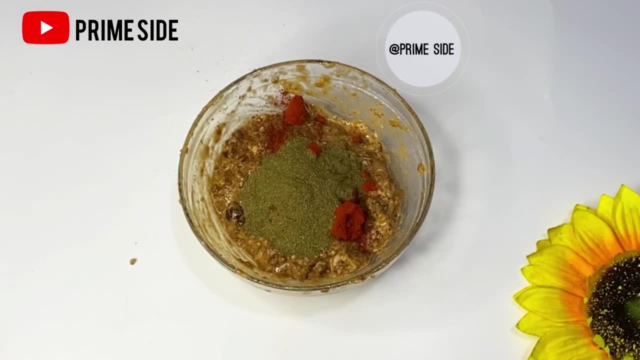 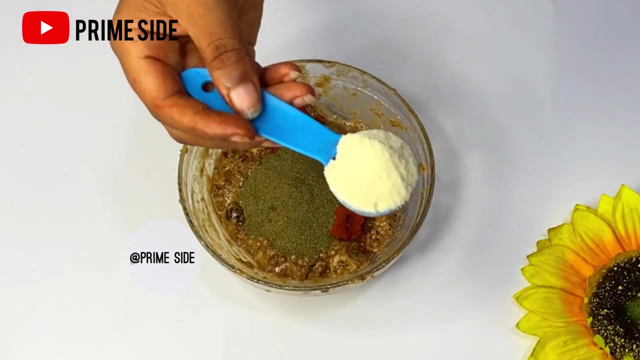 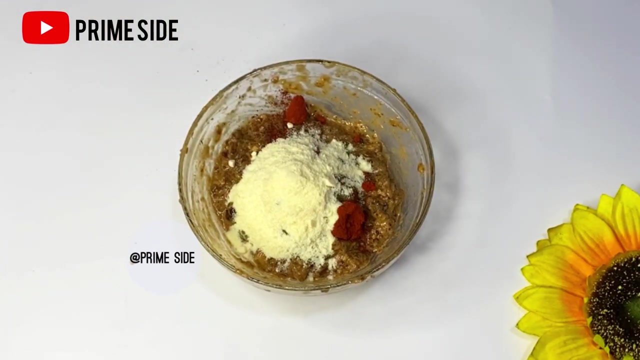 and so this will also assist the calm wood powder to make their skin more radiant and glowing, and so the next and very important powder to add to their recipe is our milk. here i'm using the goat milk powder. goat's milk is a protein that will help to nourish these children's skin and will 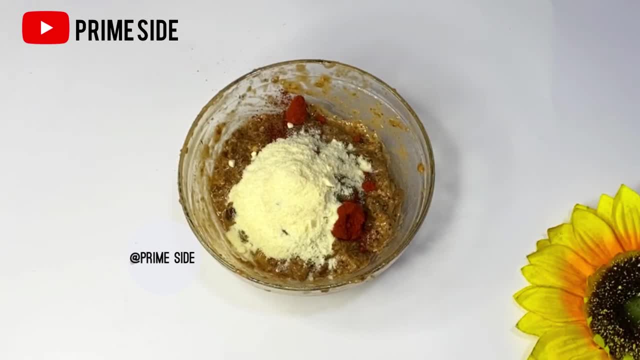 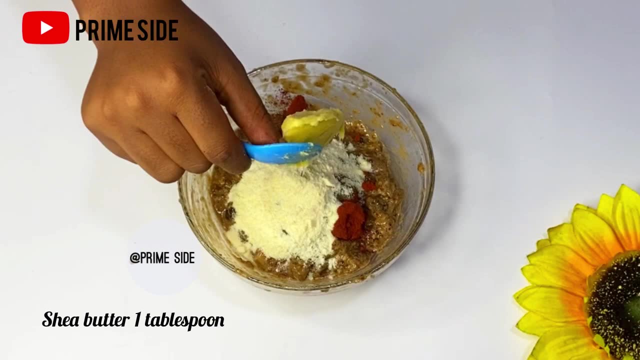 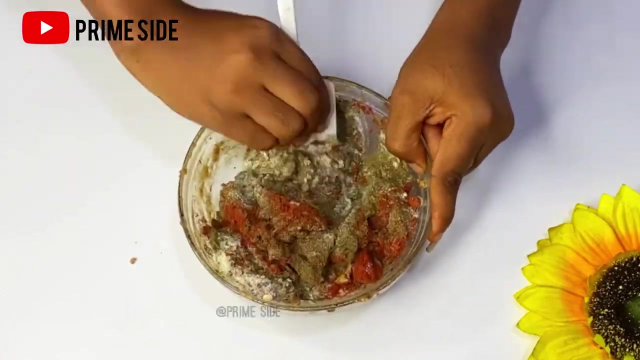 help them to have a healthy skin cells. so it is very important here you can add more than a tablespoon. also, i'll be going in with a tablespoon of sugar and i'm going to add a tablespoon of shea butter. then i'm going to be mixing these powders slightly before adding my oils. 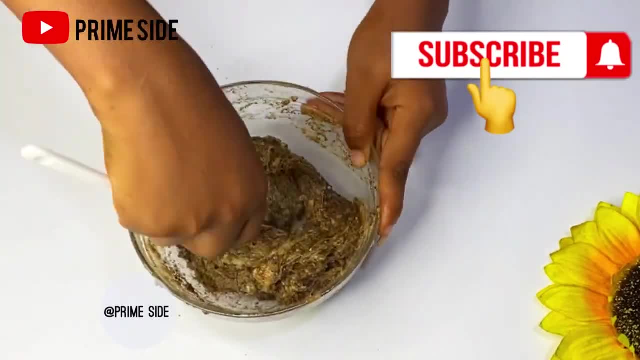 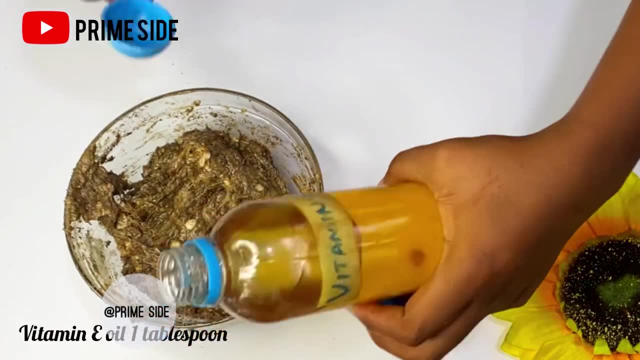 please, if you're new to this channel, help me hit that subscribe button, and if you're a returning subscriber, i know that i love you so very much, so the first oil i'll be adding here is my vitamin e oil. i recommend vitamin e oil in this recipe because of its numerous 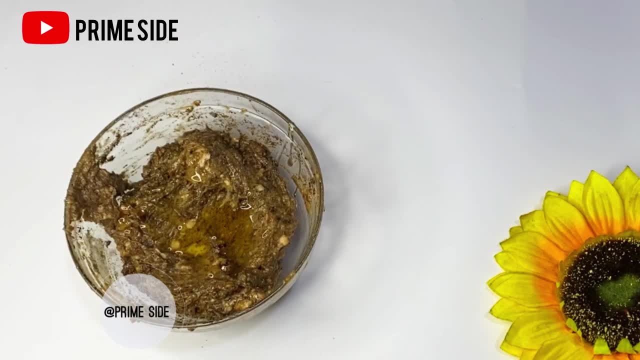 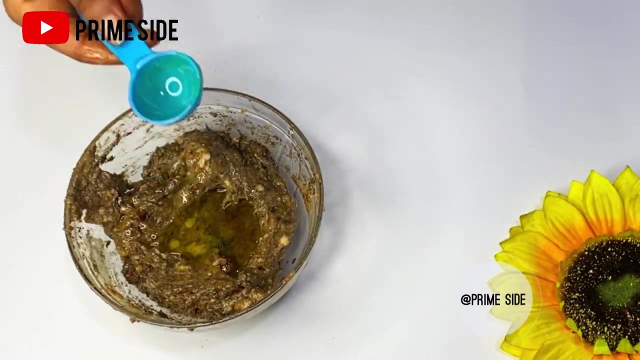 effect and because of his role in playing for skin glue. also, our neem oil will assist our neem powder inflicting bacteria and fungi conditions. the turmeric oil here will help the skin of these kids to grow. especially it will lighten up your skin a bit. and then the coconut. 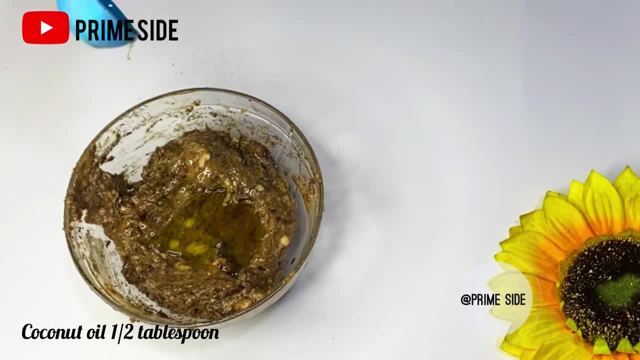 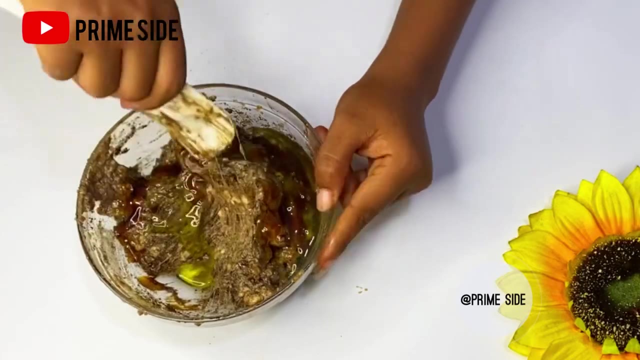 oil, or you can substitute with sweet almond oil, will also help for glowing of the skin. i'm going to add dry rolling stone, to add additional honey, because indeed these children need this natural honey for their skin, and then i will be mixing again. now, these children needs to glow, they need a nourishing skin. 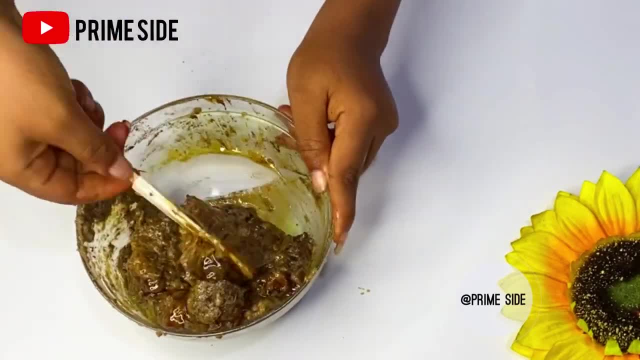 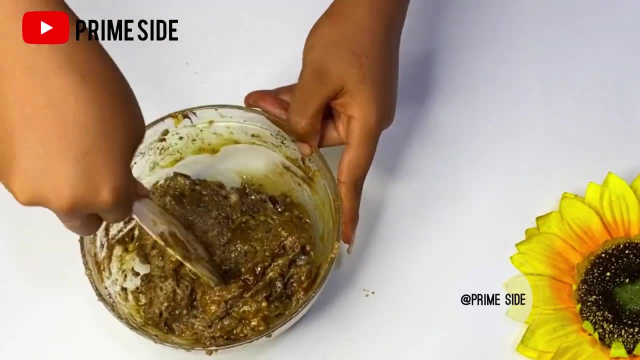 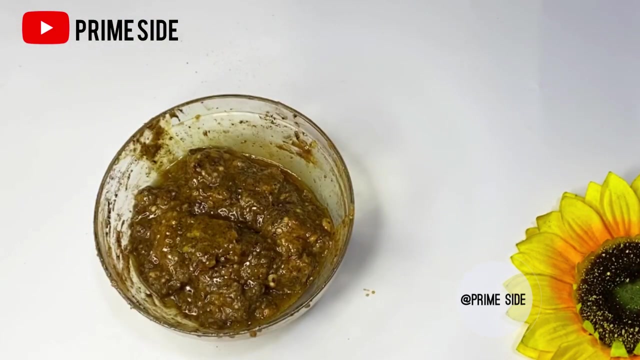 they do not need any form of chemicals to fight acne, pimples or whatsoever, and they do not need to tone their skin as well. if they are dark, let their dark skin glow, and if they are light skin, let their light skin glow as well. please do not add any bleaching agents to this recipe. 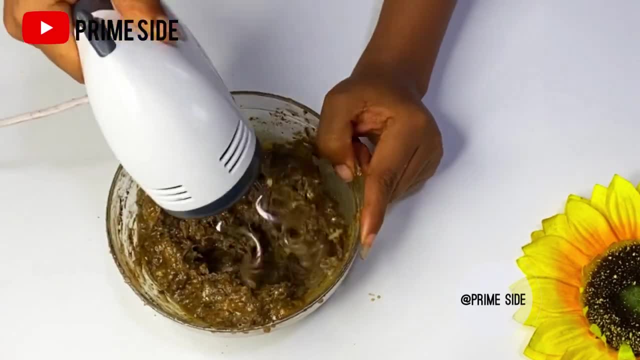 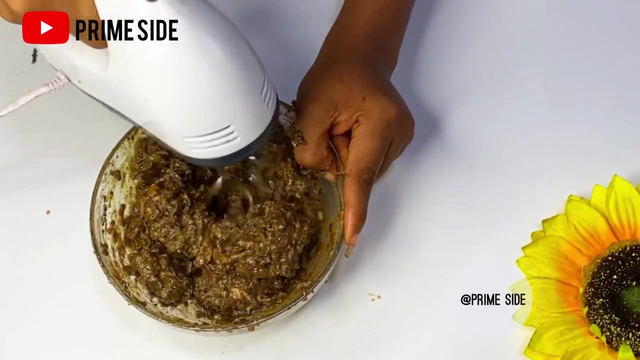 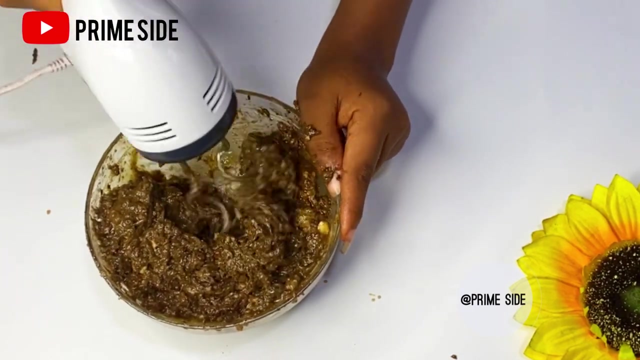 i'm using in my my hand mixer to mix this thoroughly, because i didn't use my mortar and pestle and of course it's really not smooth, but that is not an issue. i'm going to mix for a while then before i'll be adding my fragrance. 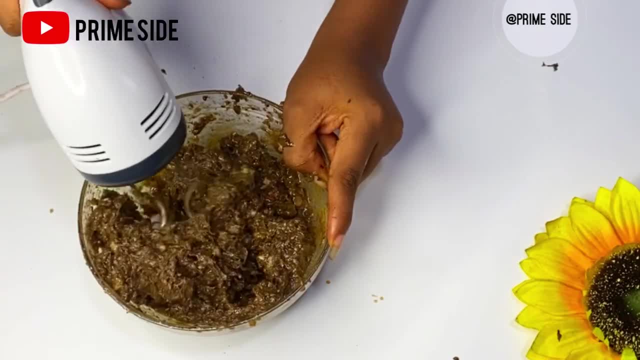 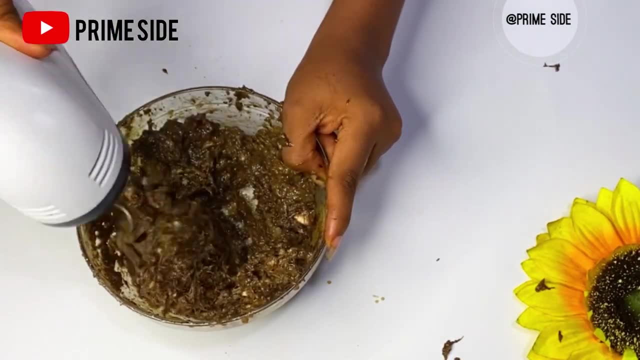 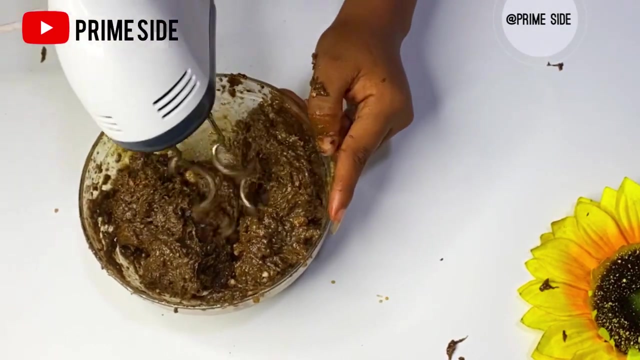 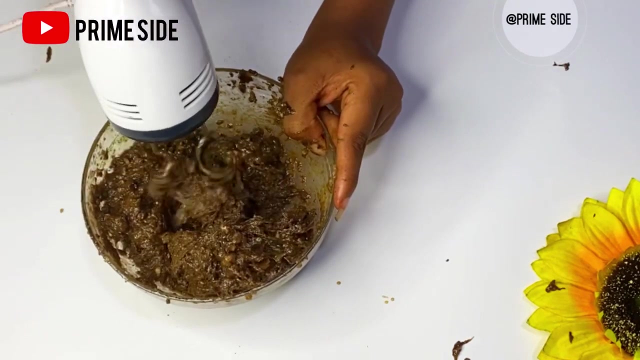 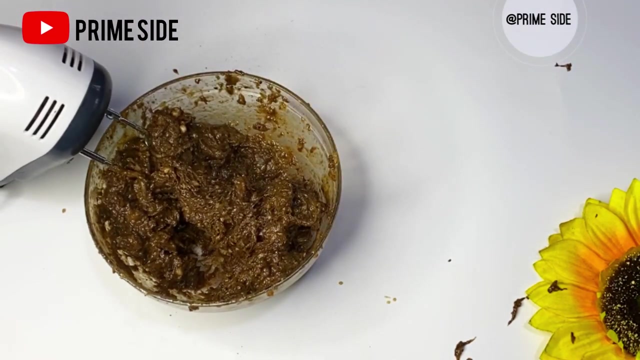 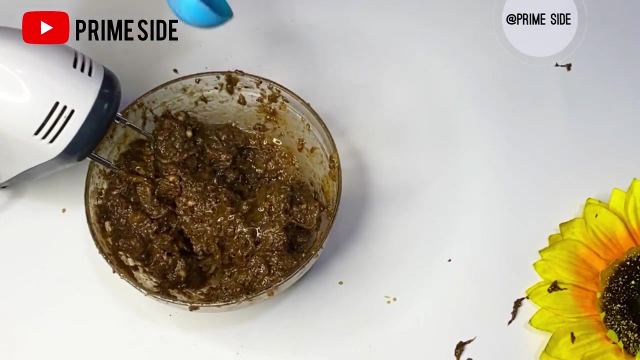 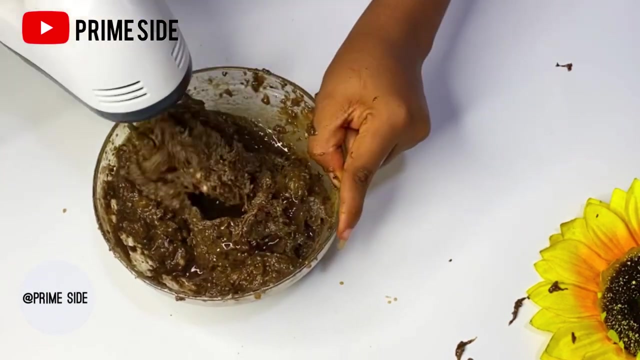 one, two, three, four, wow, soavamiy ayayaya. i'll be using strawberry fragrance for this recipe so it can smell. well, you can use any variety of fragrance that you want so the children can love this particular soup. please, and please- i'm sending it this way- do not bleach your children's skin. there is no use for that. their 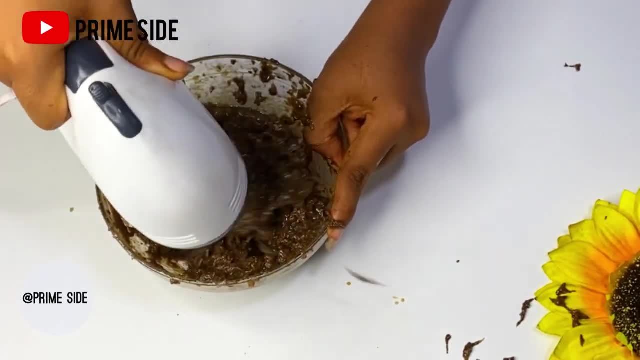 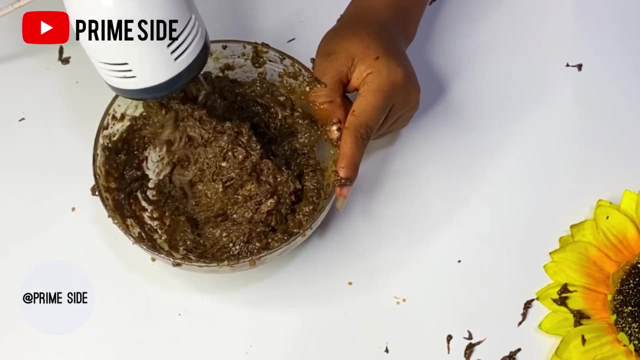 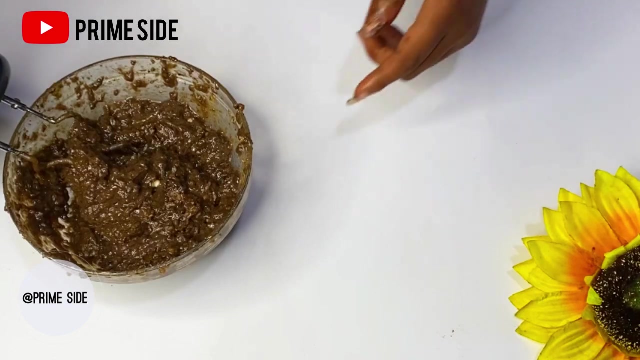 skin are too tender to undergo these harsh chemicals and what you call it natural powders, and the black soap is okay for their skin. if you want to go harder with your skin, please do not use chemicals, as it may cause damage to their skin, no matter how beautiful they may be looking.